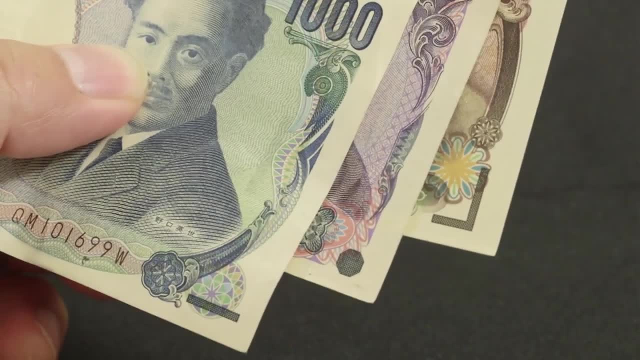 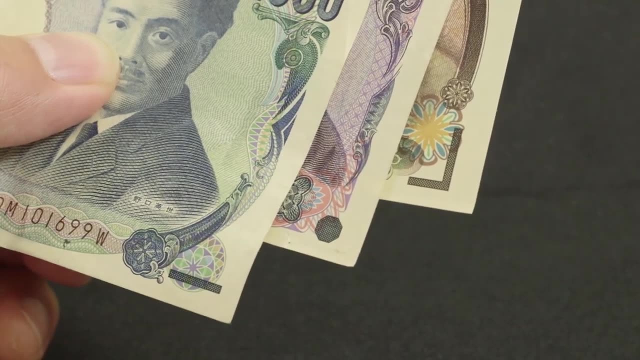 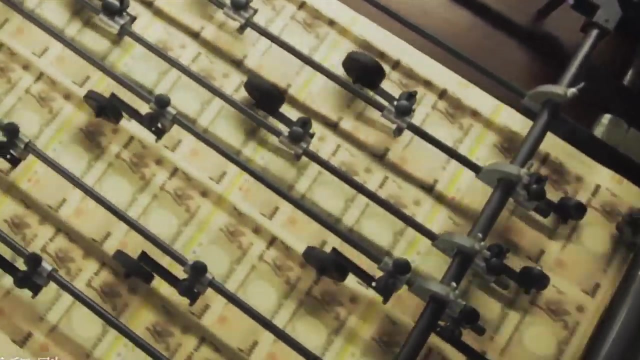 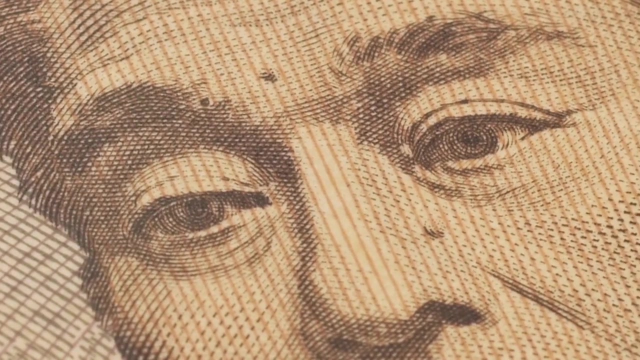 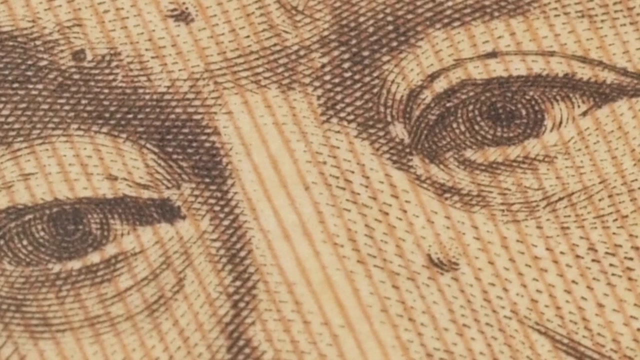 And special tactile marks printed at the corner of each banknote have different shapes to instantly convey the value of the note to visually impaired users. The most important technologies in currency manufacture are those to prevent counterfeiting. To make them harder to forge, many of the lines in a banknote design are printed narrower than a human hair. 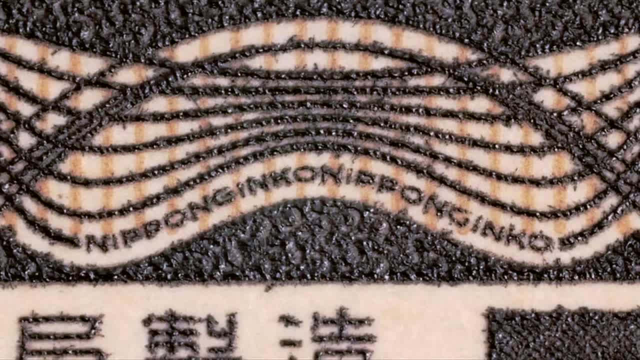 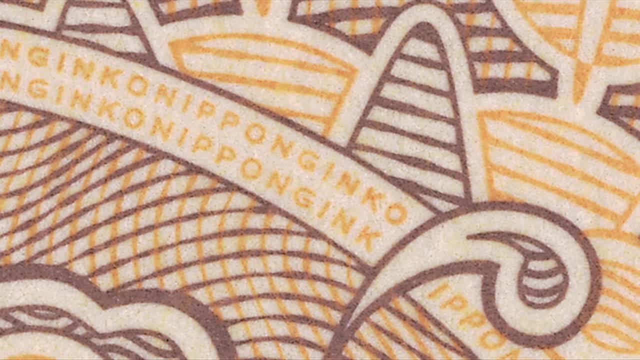 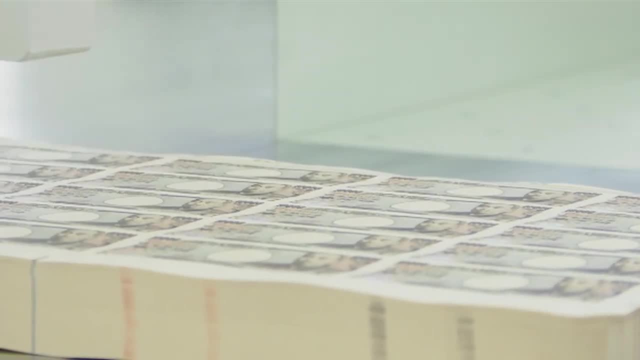 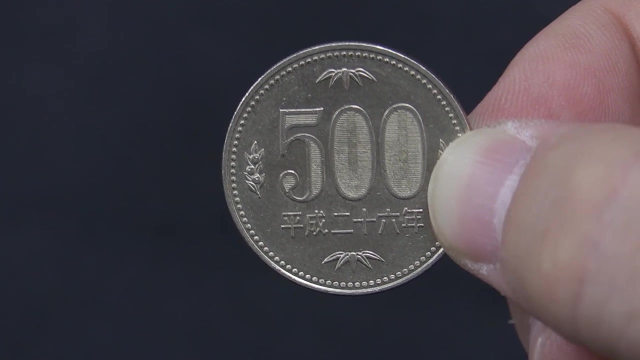 The name of Japan's central bank is printed in letters invisible without a magnifying glass. Such designs are impossible to reproduce without very sophisticated printing technology. Micro-printing techniques that produce effects invisible to the naked eye are highly effective against counterfeiters. The edge of the largest value 500 yen coin is helically milled to give it a pattern of slanted grooves. 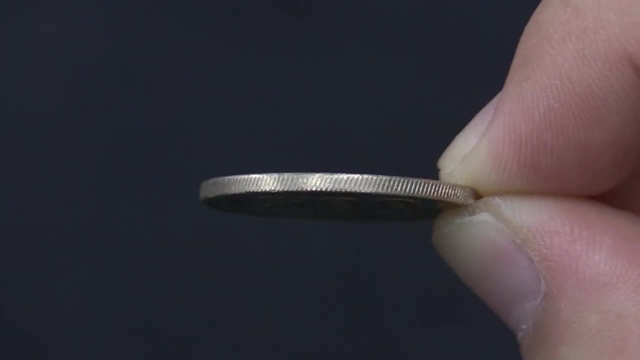 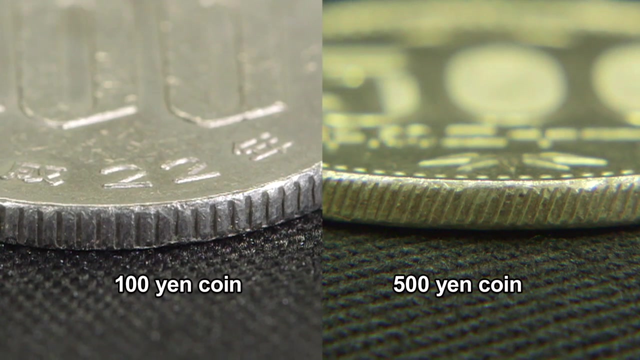 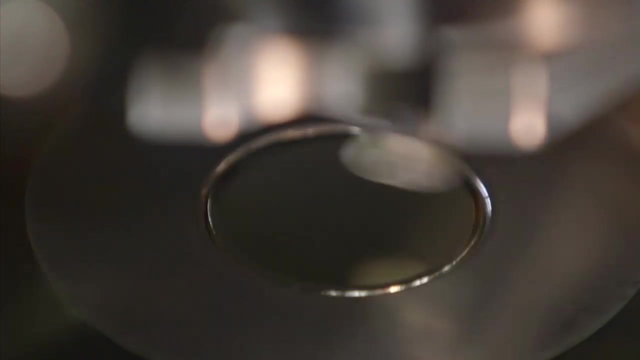 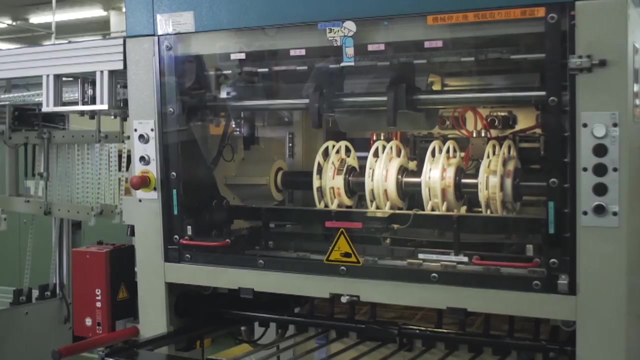 This makes the coin much more difficult to fake. Later, coins had vertical grooves that are easier to mill. The Japan Mint developed the world's first method for mass-producing coins using helical milling. This advanced technology is patented worldwide. Technological developments are incorporated as soon as feasible. 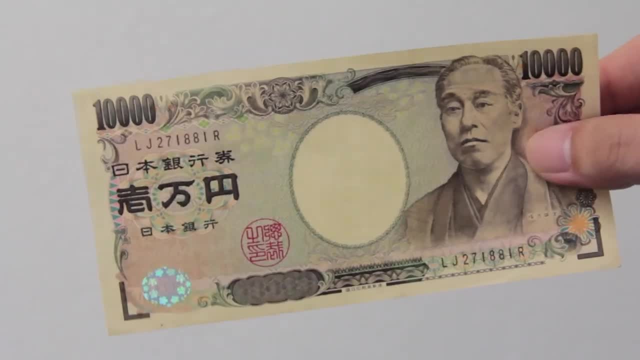 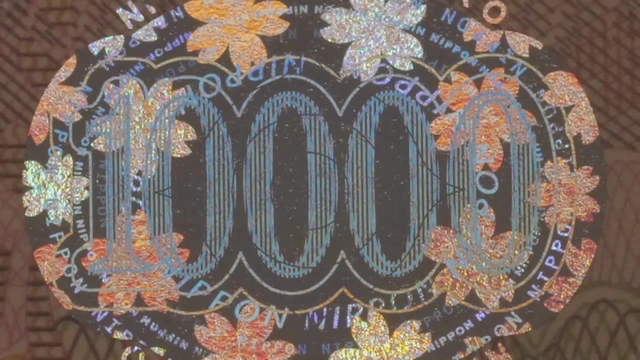 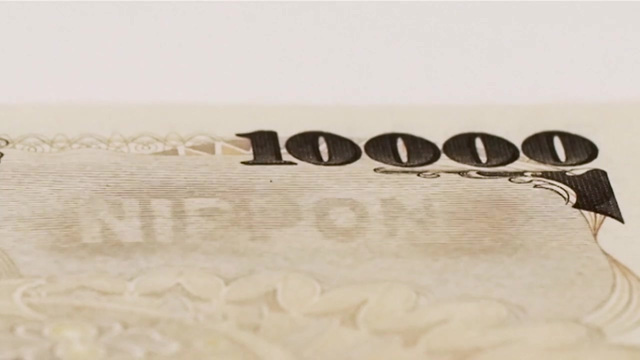 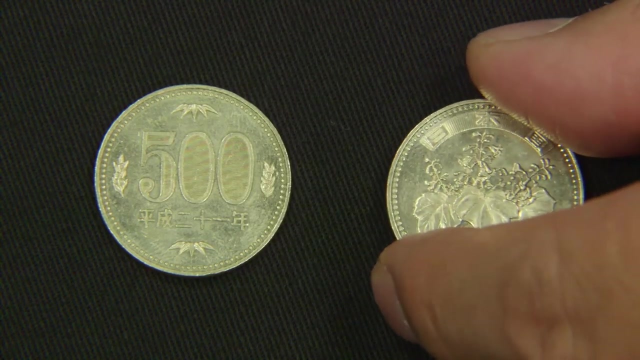 Holograms are used on the 10,000 and 5,000 yen notes. Tilt the note and the color and design of the hologram change. Tilting this note vertically reveals the word Nippon, meaning Japan. Similar technology is used for coins. 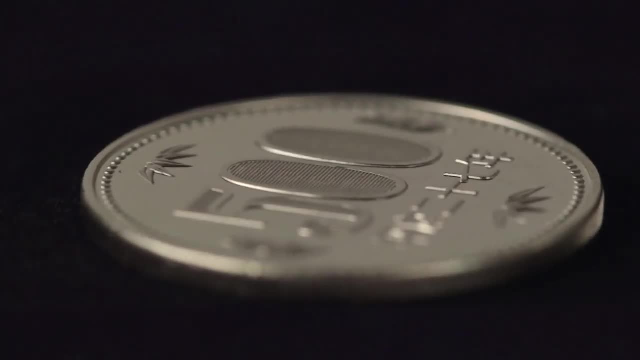 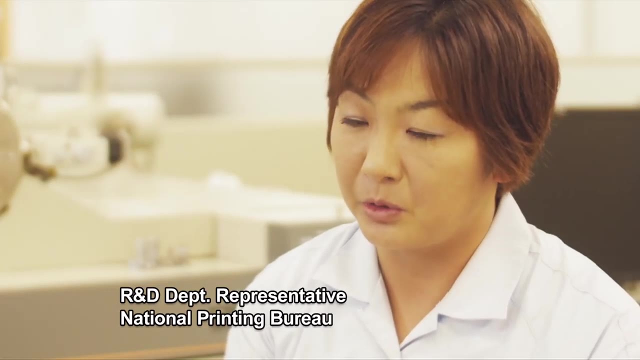 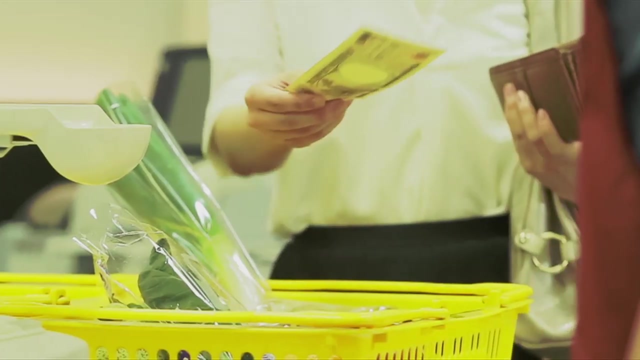 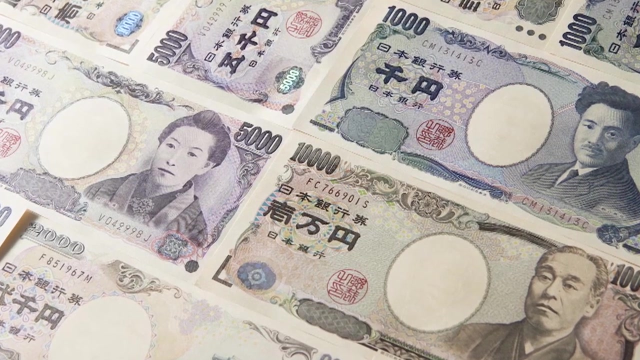 Changing the angle of view reveals hidden writing in the zeros. The color of the letters is changed. To make one of our products requires a combination of technologies and skills from many different specialists. We use very advanced anti-counterfeiting techniques in the manufacture of Japanese banknotes.